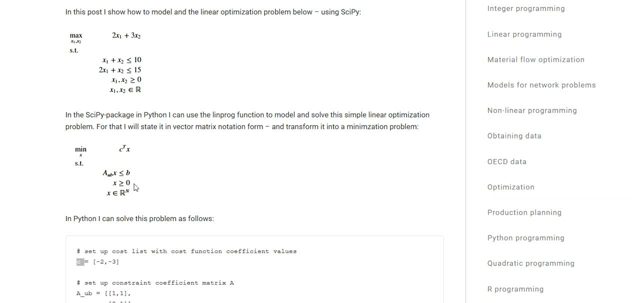 form that linproc is using or is assuming. And we can do that by simply multiplying the objective function with minus one. Then we need to describe the problem with vectors and matrices. So we need a cost vector with the coefficients of the objective function. We need a function. 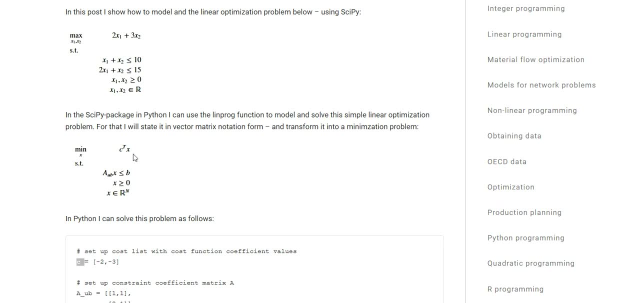 with. we need a vector with all the variables, So all of our optimization variables. Then we need a matrix with all the coefficients of our constraints And we need a constraint vector with all the values of our constraints. And then we also need to describe the lower and upper bounds of our optimization. 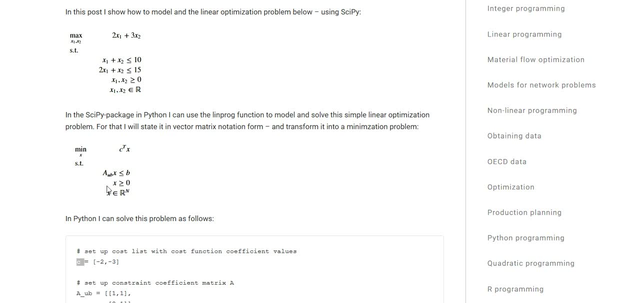 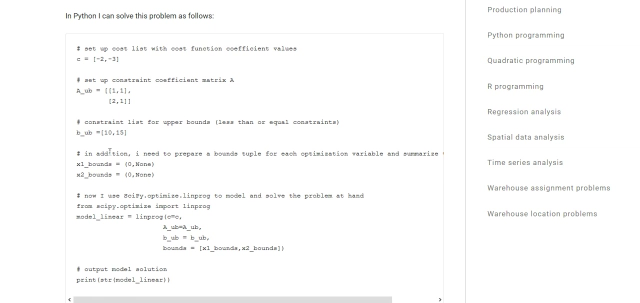 variables. In this case we do not have any upper bounds, but we do have a lower bound, which is zero. So if we go down, I'm showing here how to solve this example using the linproc function in Python And if you would like to, you can click the link in the 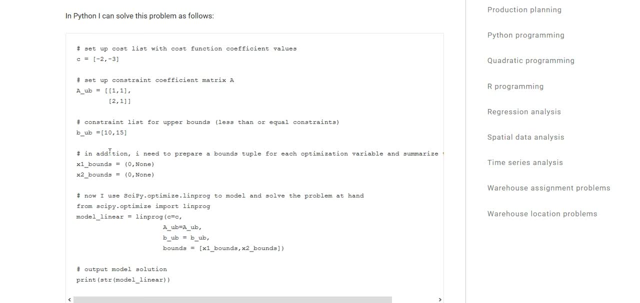 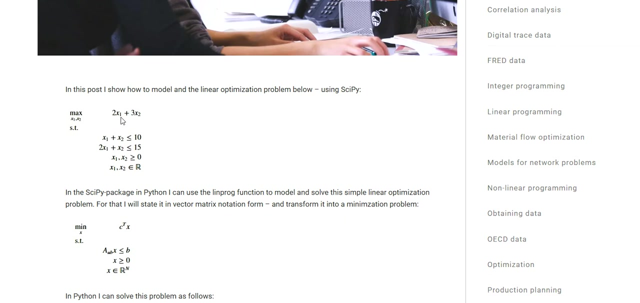 video description and see it on your own on my blog. So the first thing I'm doing is I'm defining the cost vector. Now you see, here I'm writing minus two and minus three. If you look at the original objective function, it was 2x1 plus 3x2.. But this was a maximization. 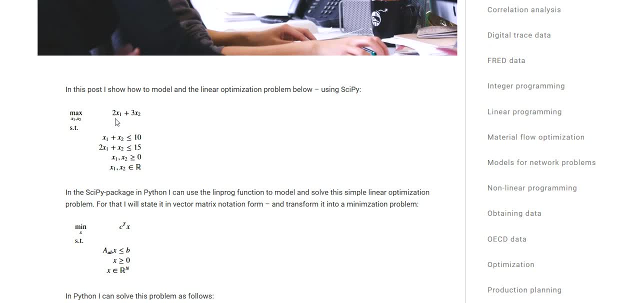 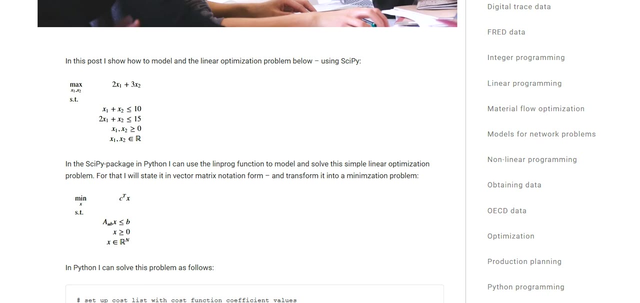 problem. We still want to solve the maximization problem, but we have to state it as a minimization problem. And we can do that by minimizing over the same objective function but multiplying it with minus one. So basically, instead of plus two and plus three, I have to write minus two and minus three. I'm now. 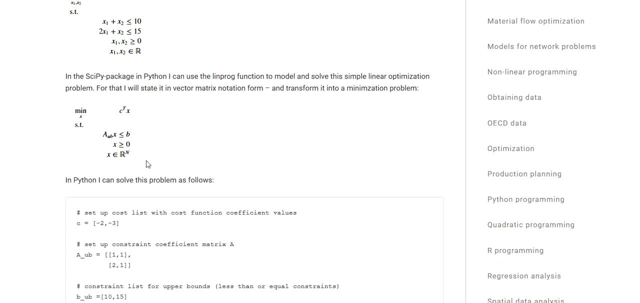 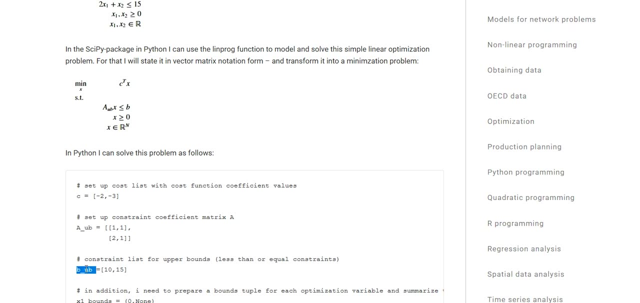 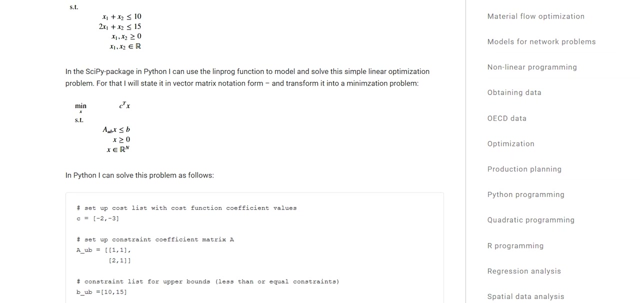 defining the coefficient matrix with the coefficients of my constraints. So my constraints coefficients are one, one, two, one. I need a vector with the constraint values which are, as you can see, 10,, 15.. And then need two tuples: One tuple for each optimization variable and the 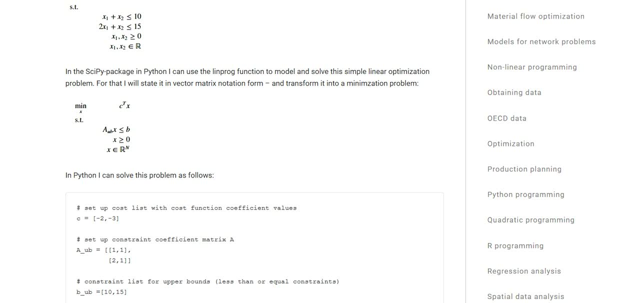 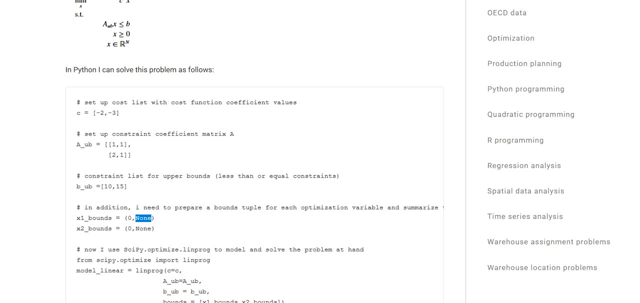 tuple will have its first entry, the lower bound, and a second entry, the upper bound. In this case we do not have any upper bounds, so I write none. Then I import the limproc function from scipy and I pretty much feed this information to it in form of parameters. So the first thing I provide is the cost. 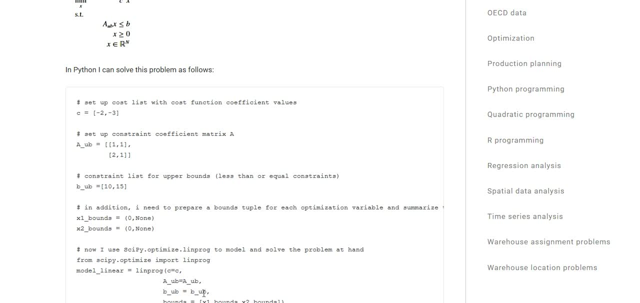 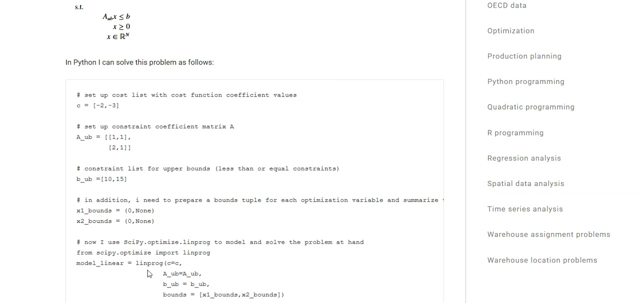 function, then the coefficient matrix, then the constraint vector with the constraint values and then a list with all the tuples that contain the lower and upper bounds for each optimization variable. And when I, once I, execute the limproc function, it will return an object. I save it here as model. 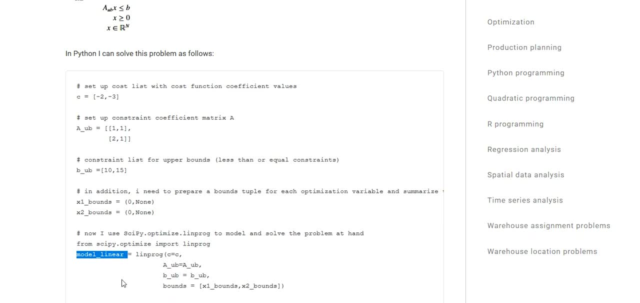 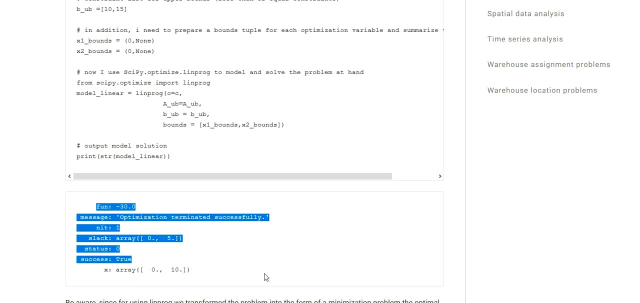 linear, because this will basically be the solution to our problem And, as you can see, I can also print this, the solution, and you will get it printed out in this form. So we can see now here the optimal solution. So this is the optimal objective function value. You can see the slack of the constraints, So you can see. 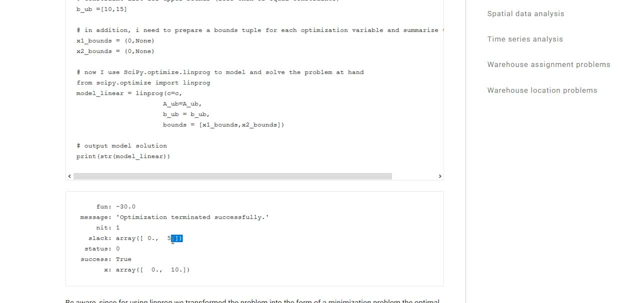 in this case the first constraint is binding. The second one has a slack of five And you can see the optimal point in our solution space here at the bottom of this printout. So x1 should be equal to zero and basically everything should be put into the second optimization. 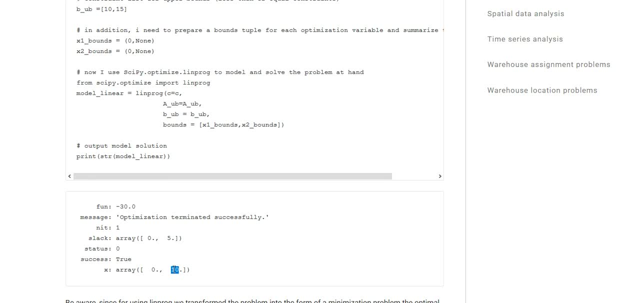 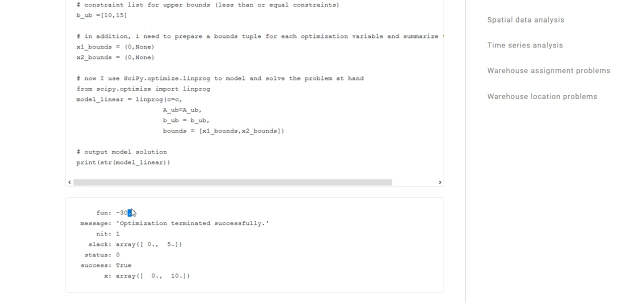 variable which is x2.. So x2 equals 10.. That would be the optimal solution. Now, the optimal value to our original problem, which was the optimization problem in form of maximization, is of course not minus 30, but plus 30. And the reason is again, in order to transform it from a 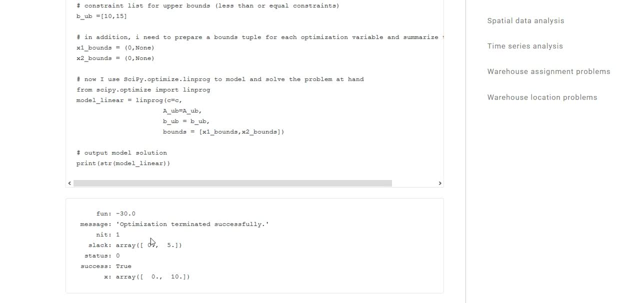 maximization problem to a minimization problem. we multiply it with minus 1.. Now if we want to interpret the results, we of course have to multiply with minus 1 one more time. So the optimal solution is plus 30 and not minus 30..